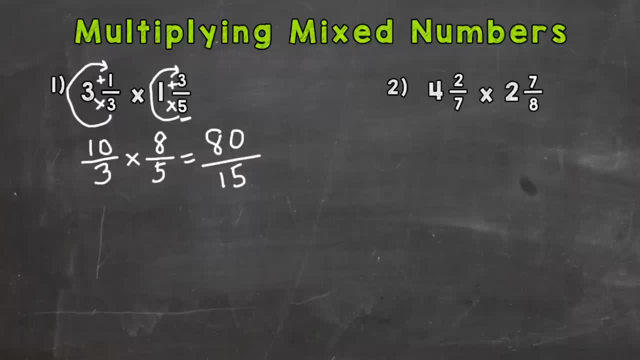 whole groups of 15 can we pull out of 80?? So I'm going to come down here to the bottom and do a division problem. Some of these you'll be able to do mental math, Some you might need to write out. So I know that 15 times 5 is 75.. That's how many whole 15s I can pull out of 80.. 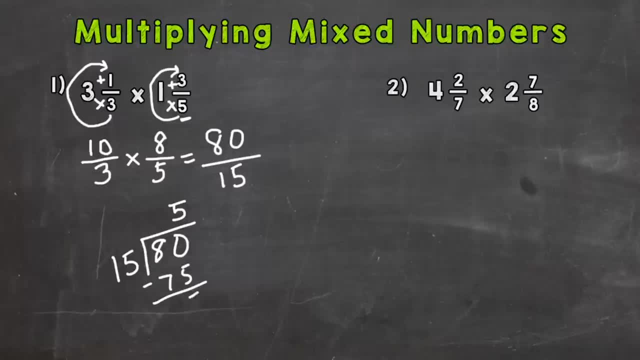 So 75 here and my remainder is going to be 5.. So the whole number for my mixed number is going to be 5.. 5 whole 15s can be pulled out of that- 80 with a remainder of 5, and I keep my denominator. 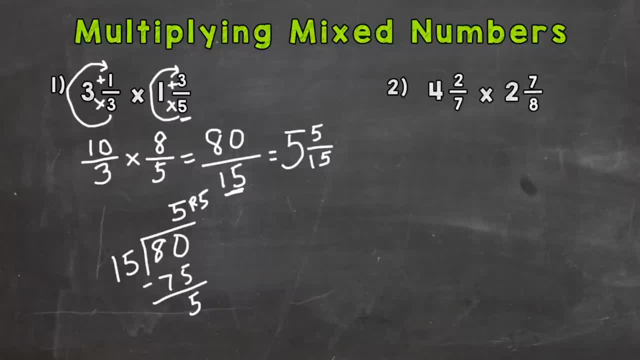 the same 15.. So 5 and 5, 15ths- and we can actually simplify that further- the fractional part of that mixed number- 5, 15ths. 5 and 15 have a common factor of 5.. So I'm going to break both of those down, divide them. 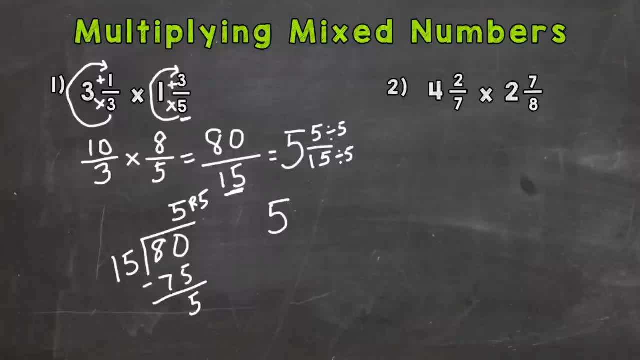 by 5.. So 5 and 5 divided by 5 is 1.. 15 divided by 5 is 3.. So my final answer would be 5 and 1. third, Let's take a look at number 2.. First thing we need to do: change to improper. 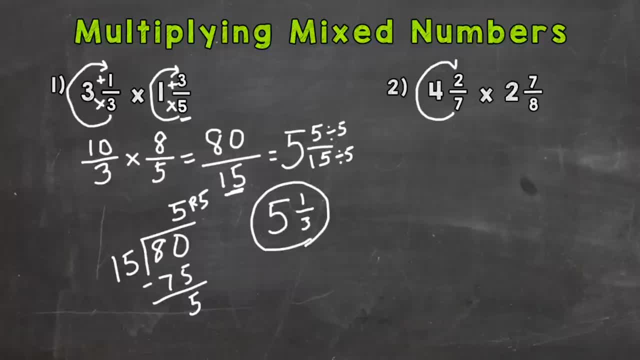 Fractions. So come around 4 times 7 is 28 plus that 2 is going to be 30. Keep the denominator of 7 the same Times. Come around here 8 times 2 is 16 plus that 7 is 23. eighths Again when you change to young. 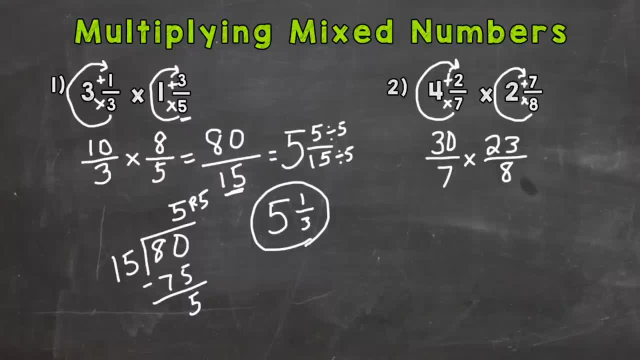 8. the mixed numbers to improper fractions. you're not changing the value of the problem or the mixed numbers in the problem, we're just changing it to a different form. now we can multiply straight across. so 30 times 23 is going to give us 690, and 7 times 8 is 56. so that's our answer in an improper.